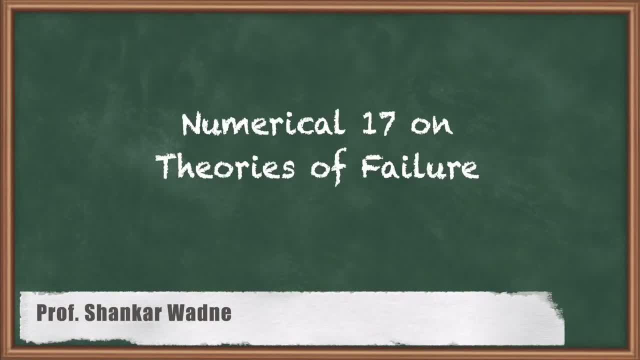 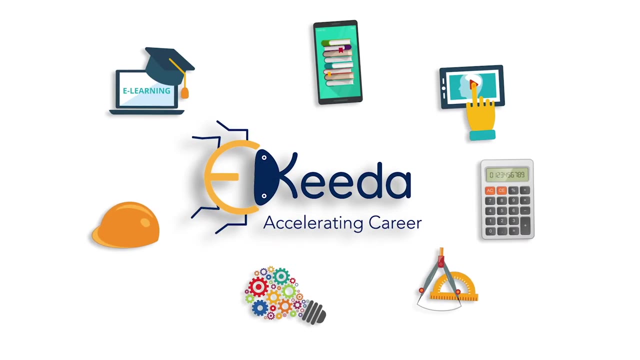 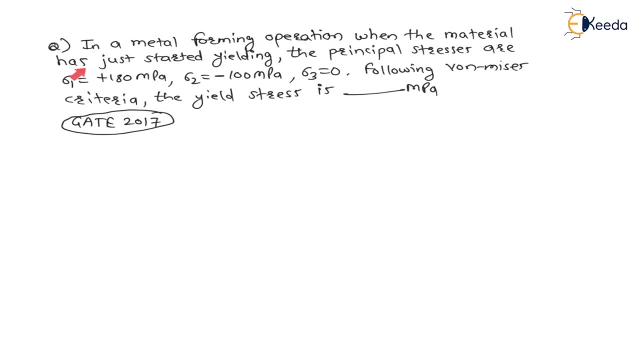 Hello, my dear students, in this lecture we will see one more numerical which was asked in previous year, GATE 2017, on theories of failure topic. The numerical is written on the screen. the question is: In a metal forming operation, when the material has just started yielding the principal stresses? 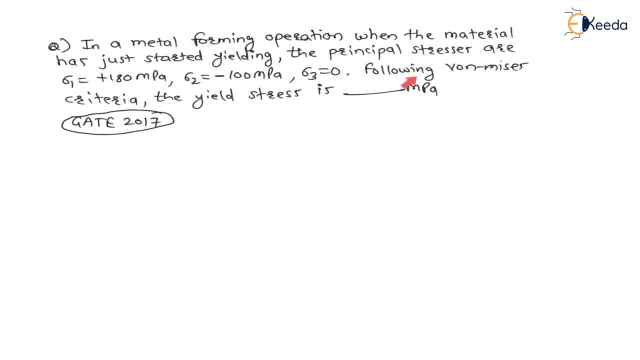 are given Following von Mises criteria, the yield stress in EMPA is- and this is a fill in the blanks question- whatever may be the answer, you have to type this answer in provided space or in bracket. And once you type this answer, 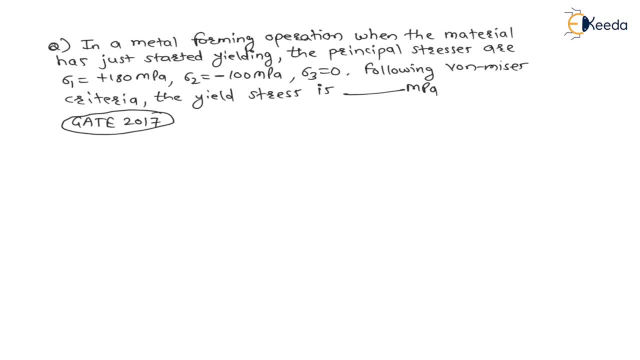 there will be no negative marking. For such type of questions, there will be no negative marking And for multiple choice question, there will be a negative marking. Now, in a metal forming operation, this is one of the metal working operation for mechanical students. Whether you are a civil student, there is no problem. 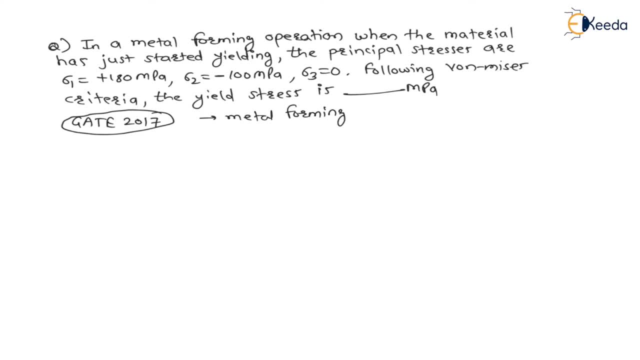 For civil students also. the solution to this question is no problem, because they have again. they have mentioned that the material just started yielding. In metal forming operation material always starts yielding. just start of yielding is written. just start of yielding. that means yielding is already started. 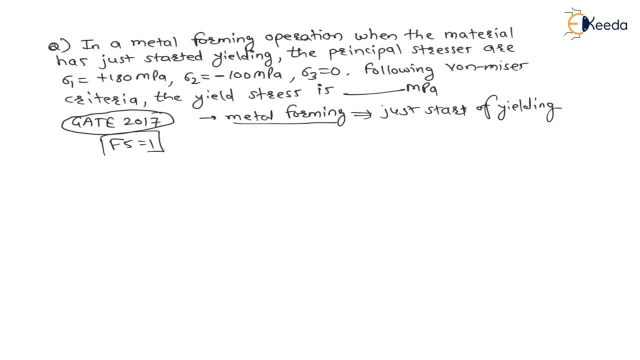 that means here factor of safety is considered one. here factor of safety is considered one. whenever yielding starts, then factor of safety is one. or whenever the operation is from the production subject. there, always factor of safety is one. right now again, the principal stresses are: sigma 1 is given plus 180 mpa, sigma 2 is given minus 100 mpa and sigma 3 is given 0. these are: 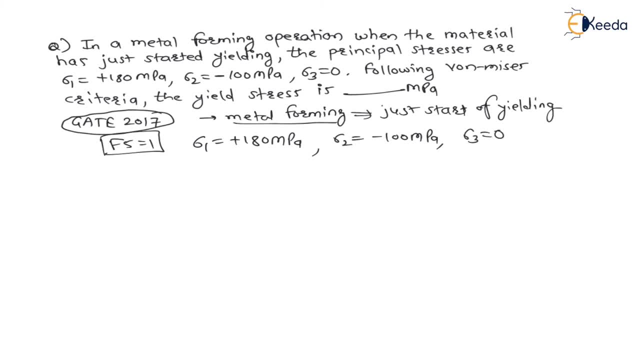 the principal stresses and following yield, following one misses criteria. the yield stress means they are asking yield stress which is nothing but s y t, stress at yield point, which is nothing but s y t. this is question in mpa and they are asking to use one misses criteria. 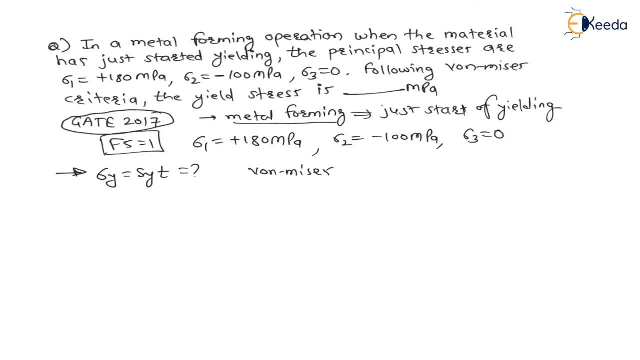 therefore, as per one misses criteria, or as per one misses criteria, or as per one misses criteria, or as per one misses criteria. as per distortion energy criteria- it is also called distortion energy, distortion energy theory criteria. the formula is: s y t divided by factor of safety is equal to under root of. 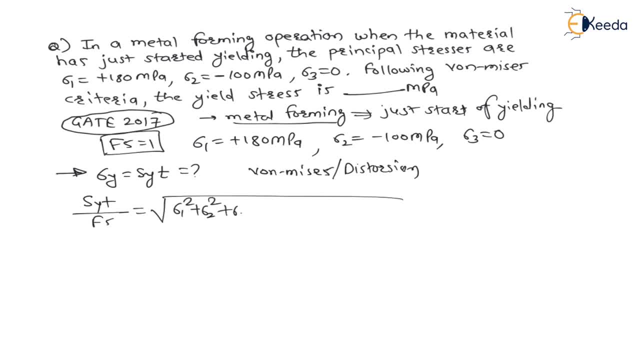 sigma 1 square plus sigma 2- square plus sigma 3 square, minus, in bracket, sigma 1, sigma 2 plus sigma 3, sigma 2 plus sigma 3, sigma 1. this formula we have to use now as already, sigma 3 is 0. 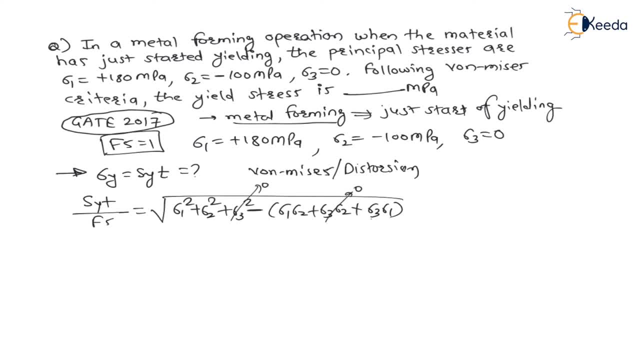